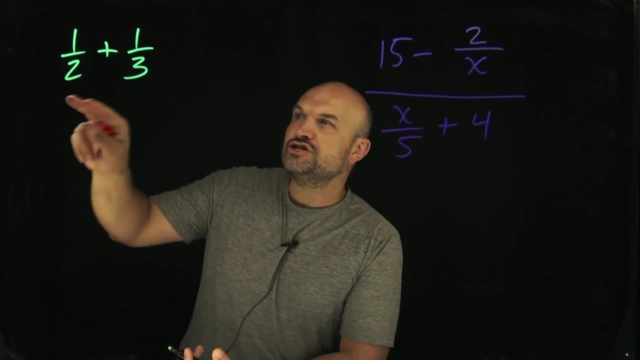 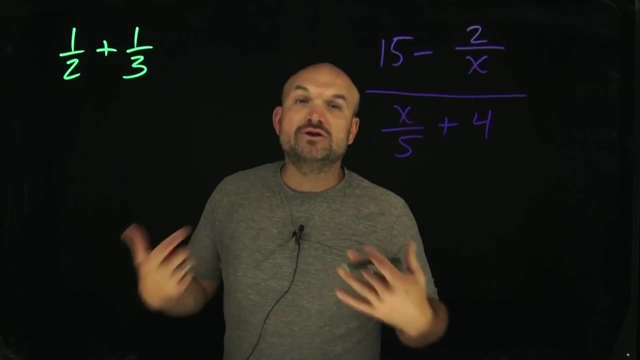 number. right, We'll call the least common denominator the smallest number that 2 and 3 evenly divide into. Now, the easiest way to be able to find a common denominator would be to multiply them. okay, And sometimes there would be like a smaller denominator that they had in. 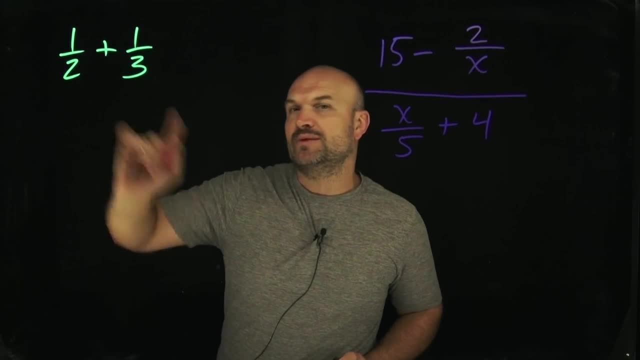 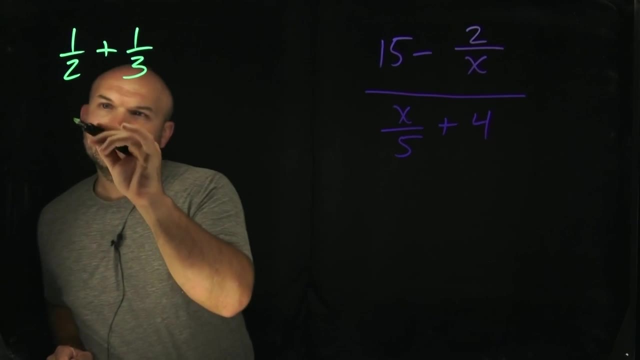 common, but a quick and easy approach that you could always work into is just multiplying your two denominators. Now, the reason why this was helpful, or the reason why this approach was, you know, a helpful way to, like, teach students about this. Actually, before I get to that, 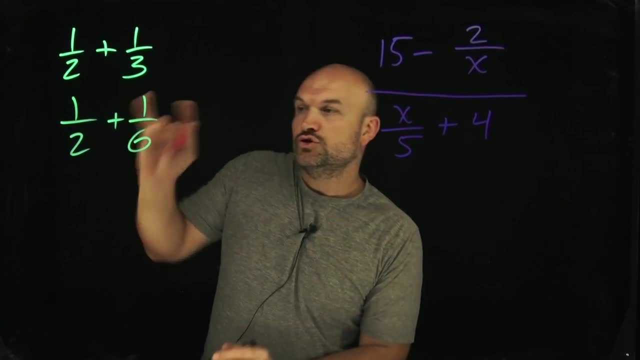 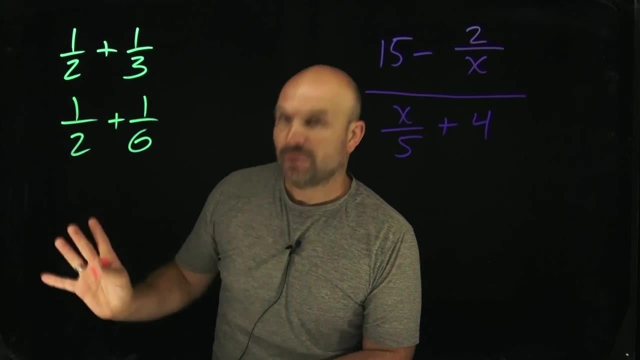 let me show you this. Like here: like, 12 is not the least common denominator, right, 6 is the least common denominator because 2 divides in 6 and 6 divides in 6.. So you don't always want to multiply them. However, the reason. 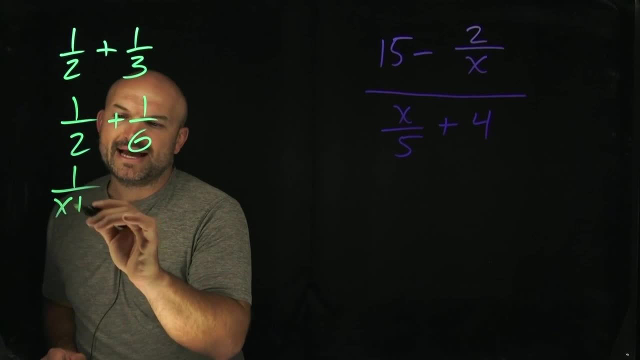 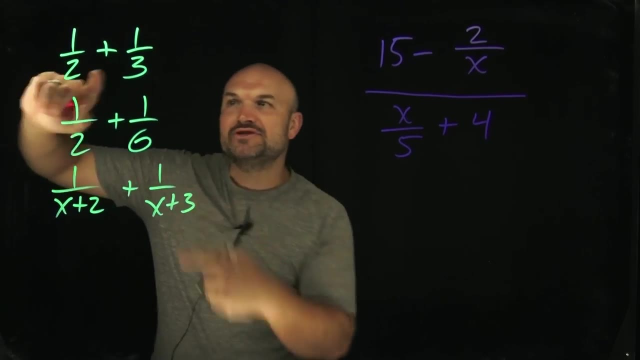 why this was important is because, like when we started doing something, like when we added expressions, a lot of students were like: what do these have in common? Like I don't know what the factors are here. Like at least with 2 and 3, we can count. like 2, 4,, 6,, 8,, 10,, 12.. Oh, 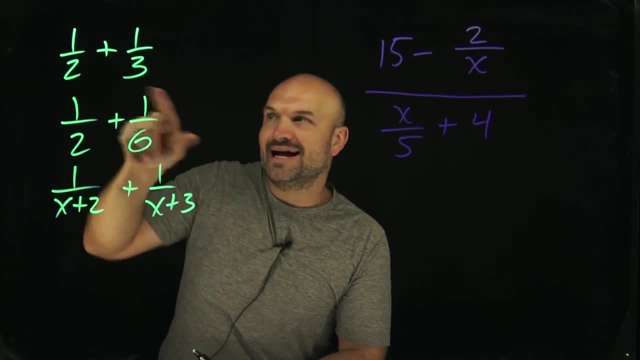 and then 6, you can do 3,, 6,, 9,, 12.. Okay, I can see what the factors are. What the heck are the factors of x plus 2 and x plus 3, right, That's kind of confusing. So what? 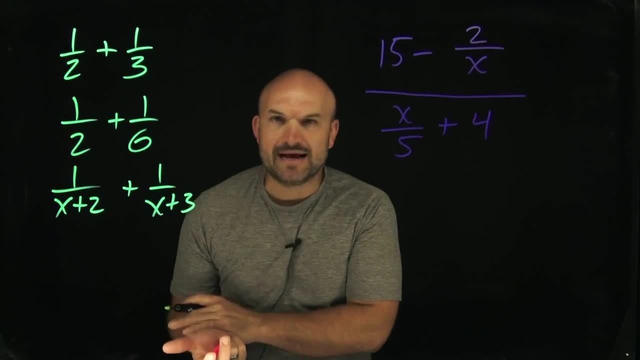 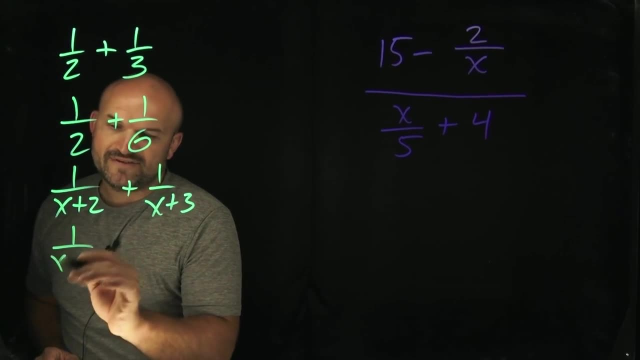 we did when we had something like this is we practiced: just multiply your denominators. Now, the only time you wouldn't want to multiply your denominators if you wanted to see if they had something in common was if you had like a trinomial where they could factor it like an x. 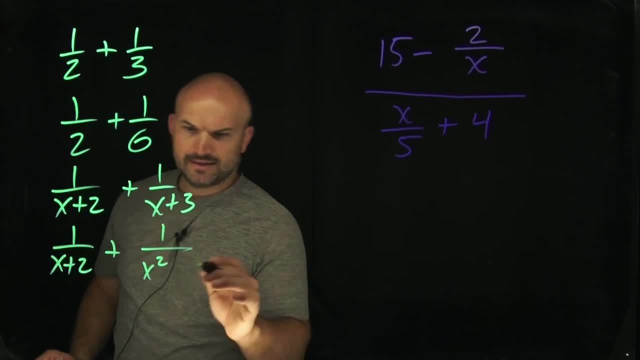 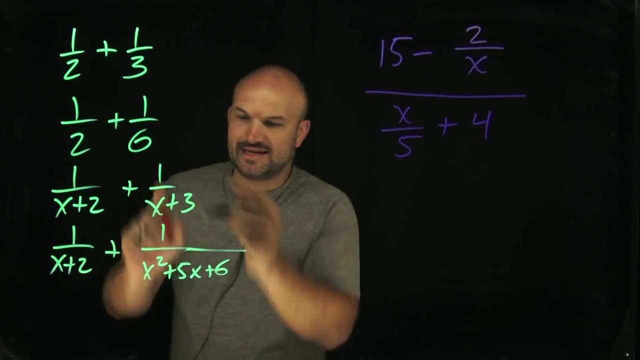 plus 2 plus, let's see, you know, x squared what? plus 5x plus 6.. So in this case, you would say: I'm not going to multiply these. What I'd want to do is just like here I want to say: well, 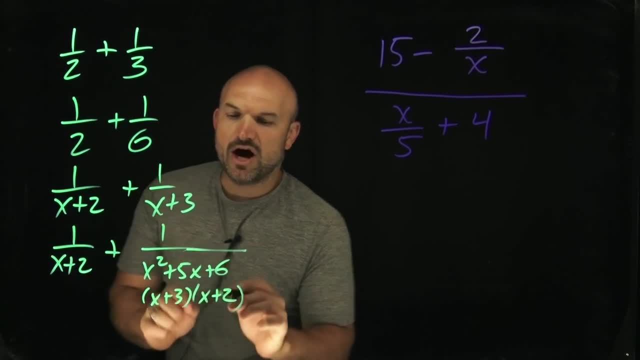 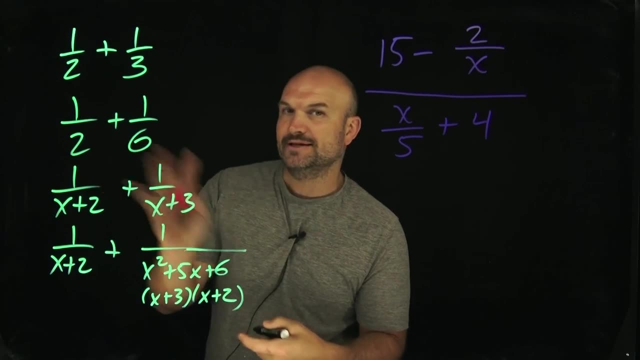 can I break this up into an x plus 3 times an x plus 2 and say, oh, they actually already share an x plus 2 in common. So therefore it's just going to be x plus 3 and the x plus 2.. All right, That's kind of like the same idea here. So let's go back and 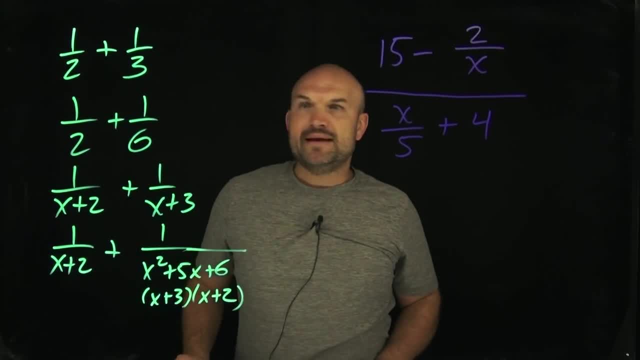 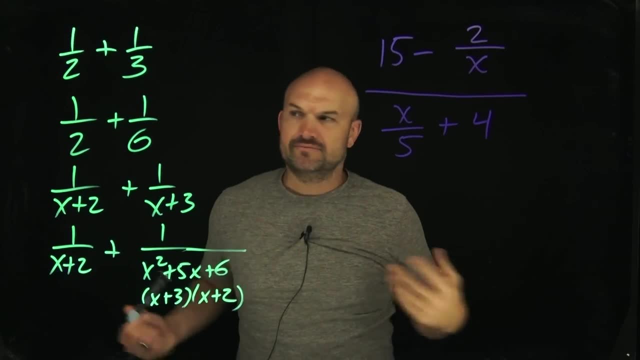 circle over to this, because why did I spend so much time talking about this? Well, my main point that I want you to understand is: I have a 5, right, That's kind of like my one denominator I got to get rid of. And I have an x. Do they have anything in common? No, right, It's like the 2. and 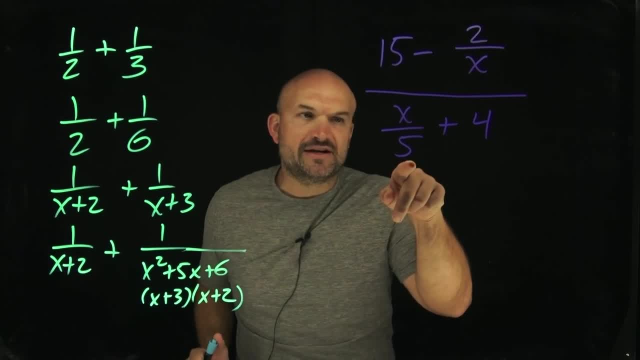 the 3. They have nothing in common. Their factors are completely different. Here's the factors that are like 5,, 10,, 15,, you know, 20,, 25, 30. Here the factors would be like x, x squared, x cubed. 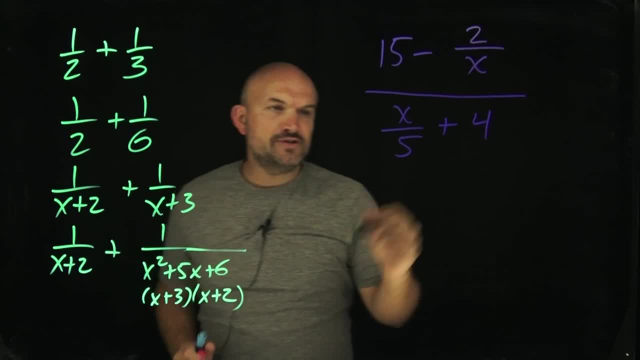 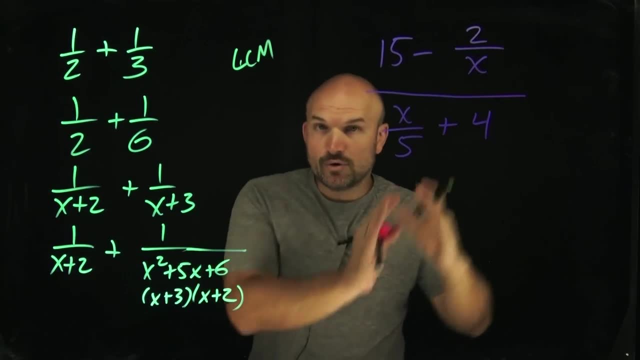 So what am I going to multiply everything by? Well, what you're going to want to do, then, in this case, is identify. the LCM is just going to be the product of the two factors. Now again, when we get into more complicated examples, we will work with factoring out your denominators. 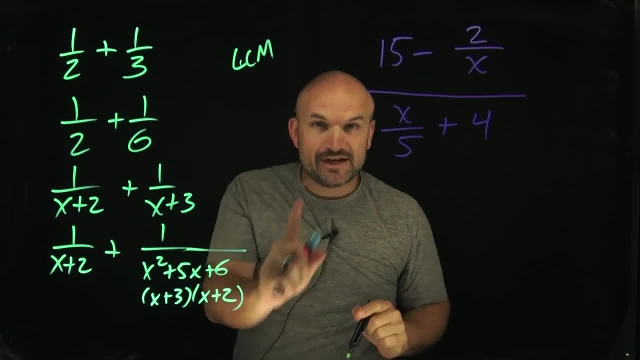 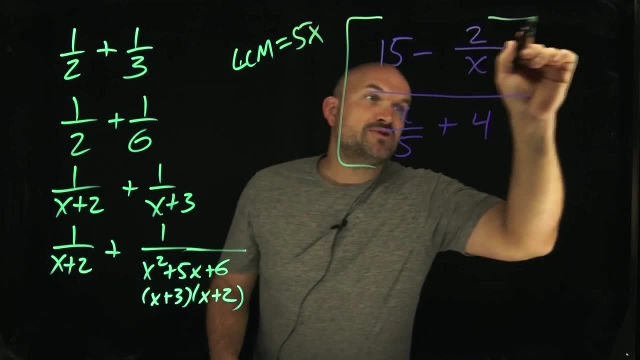 and seeing what they have in common. But in this case they can't. if your denominators cannot be simplified, then just multiply your two denominators. So, therefore, that's going to be a 5x. Now, what I'm going to do is I'm going to multiply everything times a 5x- Everything Now. 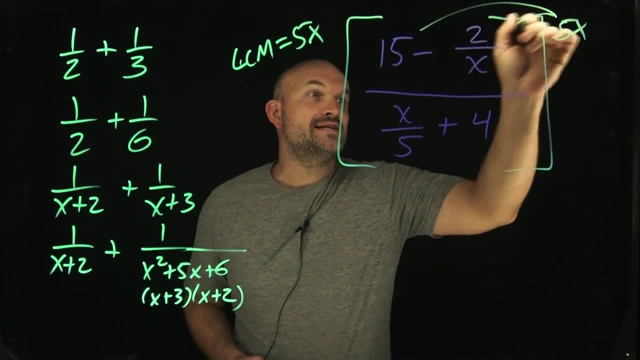 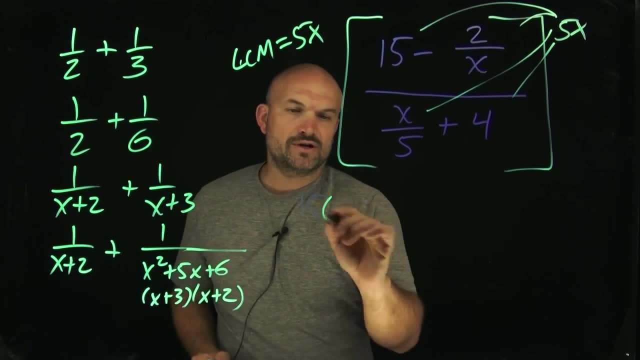 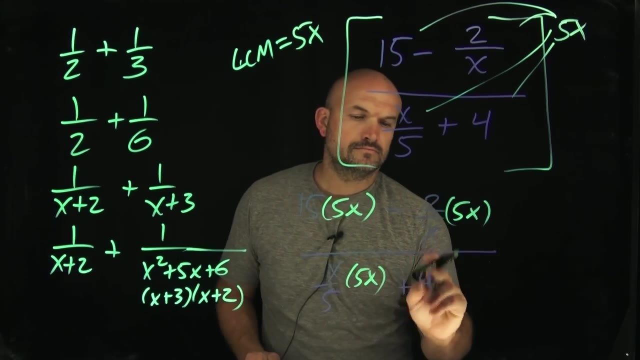 I know sometimes that can be confusing, So what I'm going to do is I'm actually going to rewrite everything times my 5x, All right, So it takes a little time, but I think it's just helpful for you guys to see how this is going to work. Okay, So now you can see I destroyed everything And 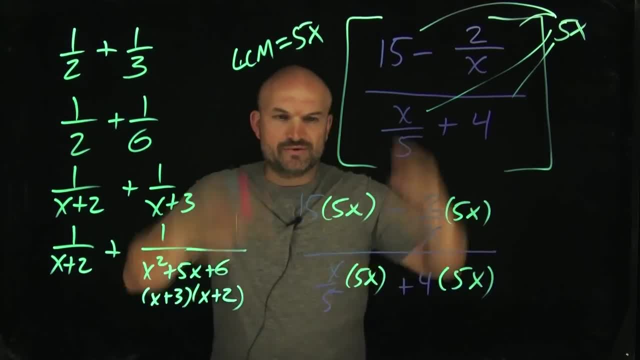 again, like, the more experience you get with complex fractions, you can start to start doing some of this in your head. You don't have to actually, you know, multiply all this stuff out. You'll get a little bit quicker on it, That's fine. 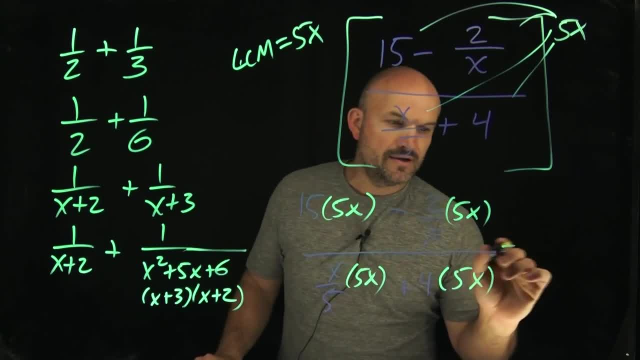 But now what we need to do is just go ahead and simplify to see what our- you know- final answer is going to be. So in this case, you can see I have a 15 times five, So 15 times four is going. 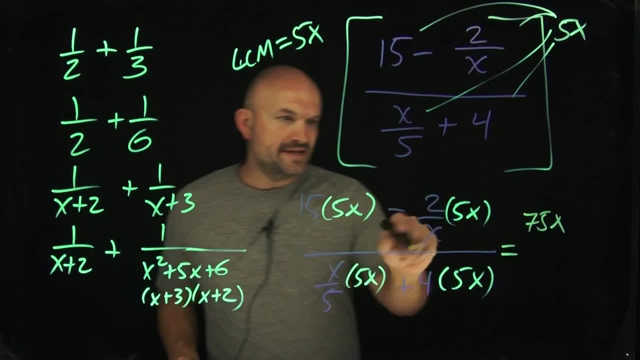 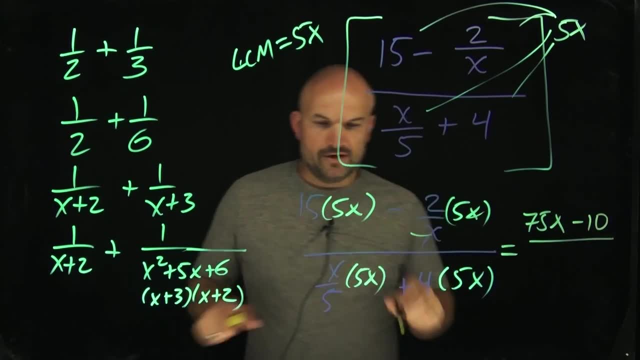 to be 60. So that'd be a 75x. And then here the x's now are going to divide out And therefore it's a negative two times five, which is going to be a negative 10.. And then over here the fives. 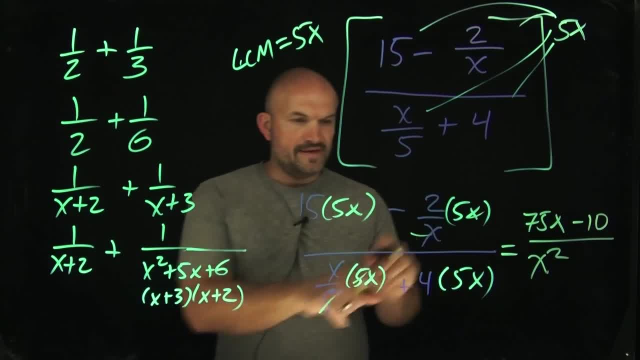 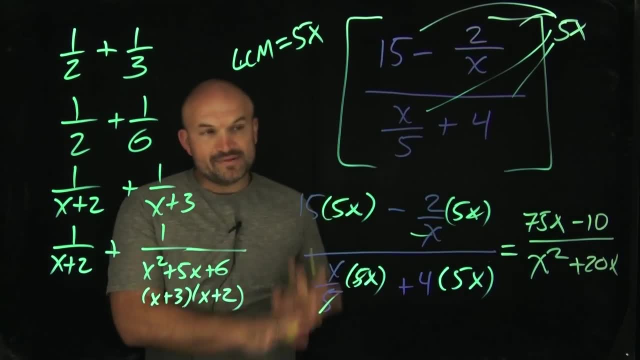 are going to divide out. That's going to leave me with an x squared, And then, over here, that's going to give me a nothing's going to divide up, but that's going to leave me with a plus a 20x. Now, if we want to be able to identify what our factors are going to be, you could factor: 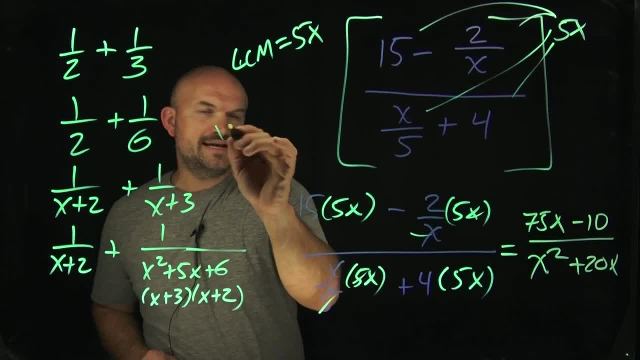 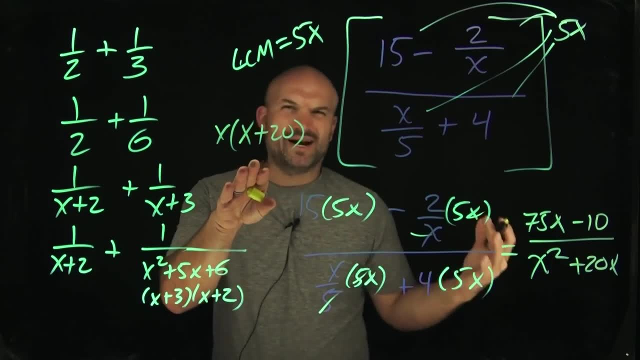 out here, So I can't really do anything with my numerator, but I could factor out an x and that'd give me an x plus a 20.. Okay, So now we know that x, so you could simplify the denominator, if you.